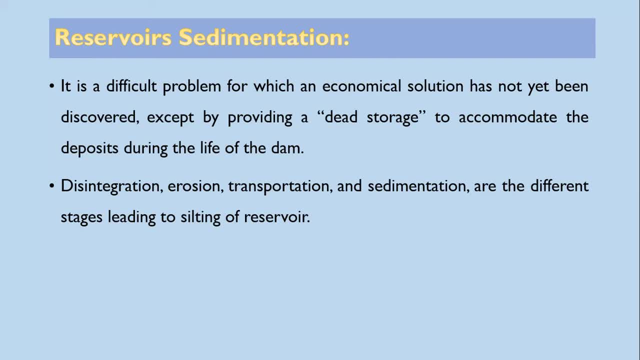 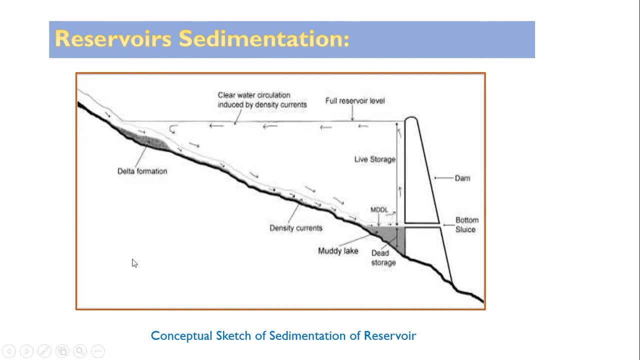 and then the reservoir capacity- Horror capacity- can be enhanced, can be improved. So here you can see the sketch. So here this stream is carrying the sediment and here you can see there is a dead storage and a muddy lake will get formed due to the streams which are carrying the sediment or suspended particles. 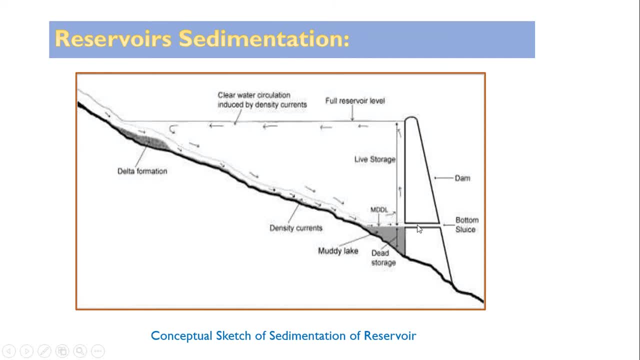 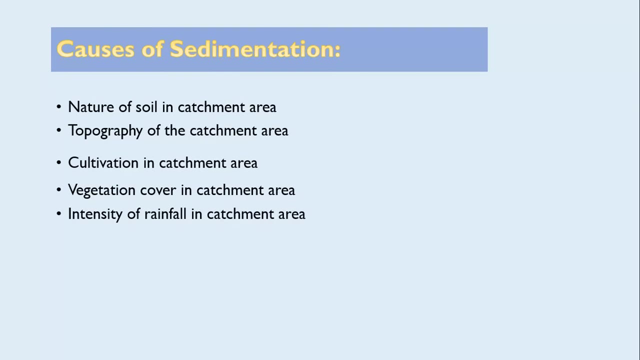 You can see the dam section. and due to this, if this amount is more year by year, the life storage will get reduced. Now, what are the causes of sedimentation? Causes of sedimentation are: nature of soil in the catchment area, topography of the catchment area, cultivation. 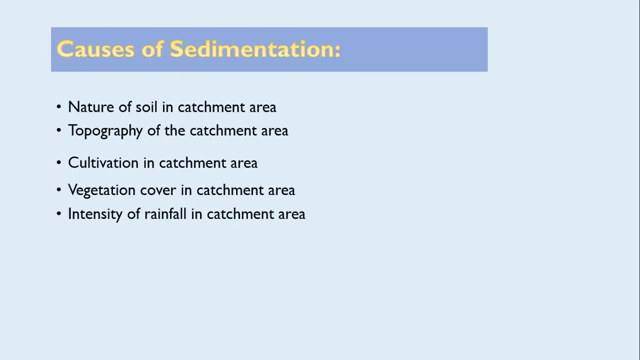 in catchment area. vegetation cover in catchment area, intensity of rainfall in catchment area. So these are the causes of sedimentation. Nature of soil in the catchment area. If nature of the soil, that is soil, is silty soil is there, the loose soil is there in the catchment area. So, along with the flow, 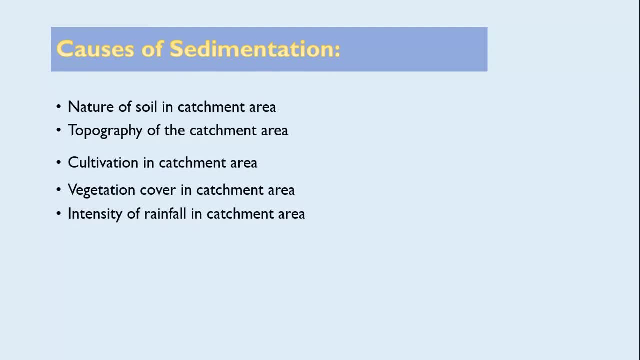 so definitely that soil will be carried to the reservoir. Topography of the catchment area. topography is nature of the ground. If topography in steep area is there, in that case during the intense rain there will be erosion of the area and the soil particles. 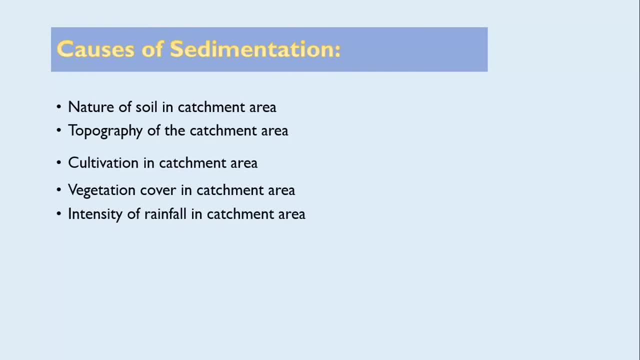 will get removed and will get flown With the plane, with the streams, to the reservoir. Cultivation in catchment area. the method of cultivation. it largely affect the sedimentation in the catchment area. Vegetation cover in the catchment area. if vegetation is dense in the catchment area, definitely it will. 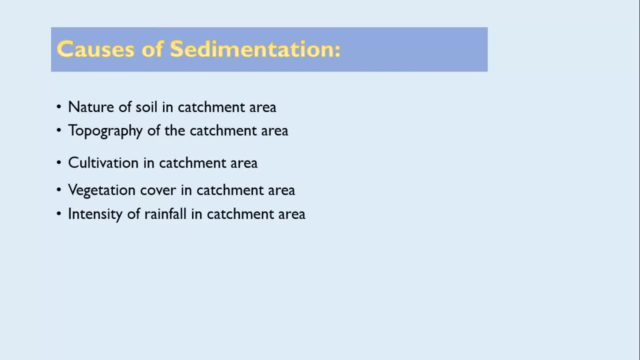 obstruct the particles to move along with the flow. Intensity of rainfall is very important. If, in the catchment, the intensity of rainfall is more, in that case there will be beating action of the soil And it will remove the soil particles and which will contribute to the sedimentation. 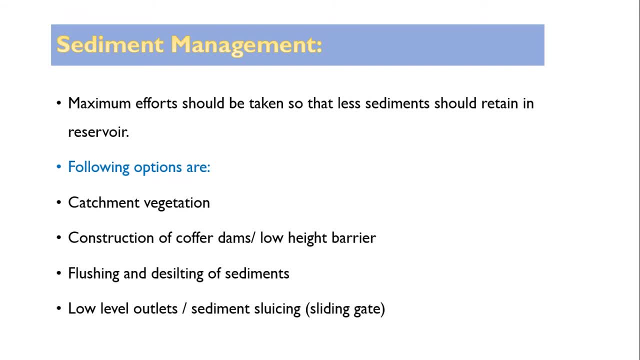 Now coming to sedimentation management. maximum effort should be taken so that less sediment should retain in the reservoir. So following options are there: catchment vegetation, construction of the copper dam, flushing and desilting of the sediment. low level outlet sediments. 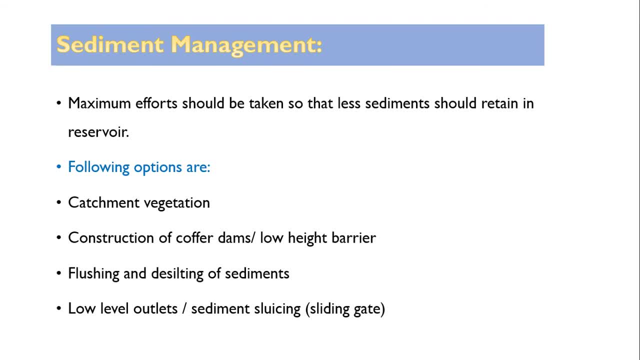 using or sliding gates. So catchment vegetation: already we have discussed. if dense vegetation is there, If there is no sediment, it will obstruct the sediment, It will reduce the sediment. Construction of the copper dams. copper dams, these are the low height dams, small dams, which 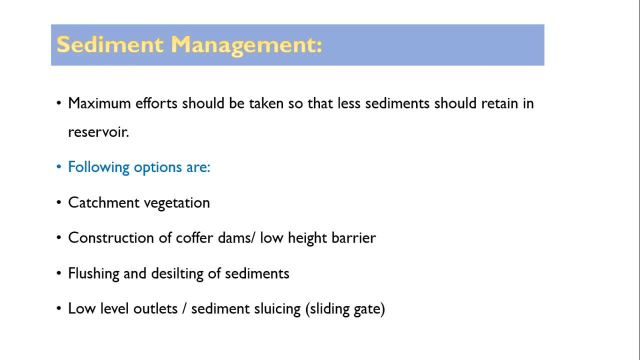 are constructed on the upstream side of the main dam And due to this, the soil particles, the sediment, it can be detained And definitely it will safeguard the main dam. Flushing and desilting of the sediment: Sediment: it can be flushed, Desilting of the sediment is possible. 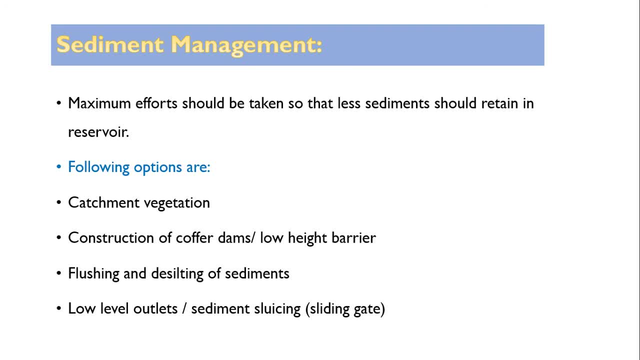 in the dam. But that's what arrangement should be Made in the reservoir: Low level outlets, sliding gates, sediment flushing, as I had explained regarding the silt excluder. that arrangement can be provided in the dam, But it is not economical. It is not economical as such. At the same time, removal of the 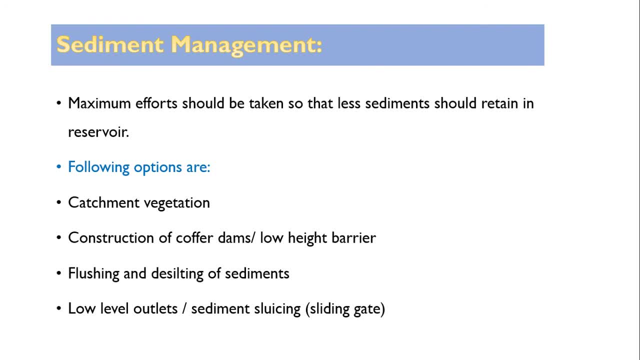 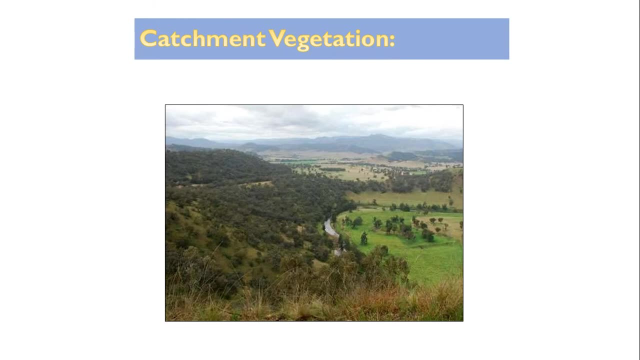 sediment from the reservoir during the dry season also not possible because it is not economical, Because the construction cost of the removal of the sediment may sometimes be close to the construction of new dams. So this is about sediment management. So here all we have discussed if this type of dense vegetation is there, definitely 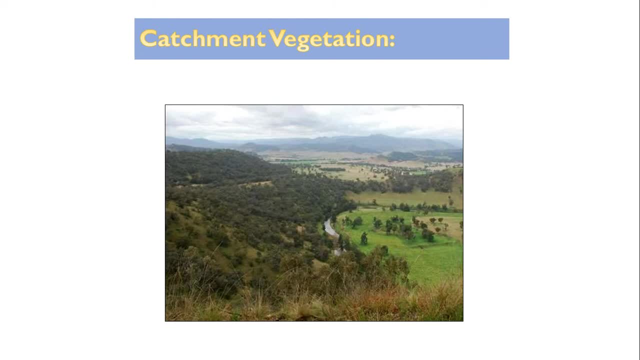 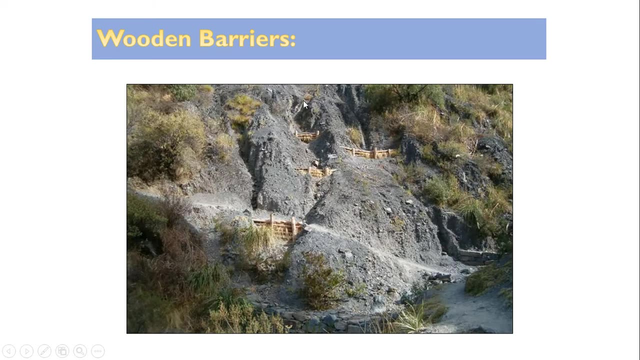 it will reduce the sedimentation from the catchment. Then here, sometimes this type of wooden barriers. these are constructed if there is a topography. stiff area is there. This is still a stiff topography. stiff slopes are there. 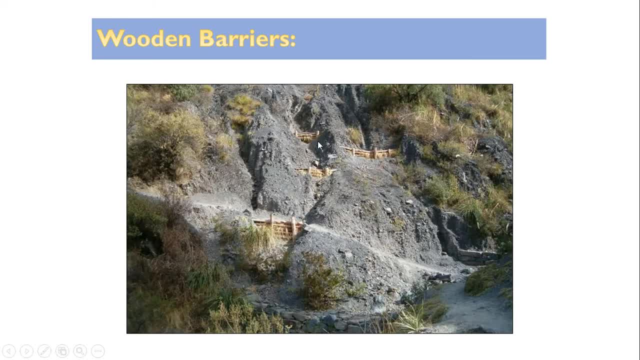 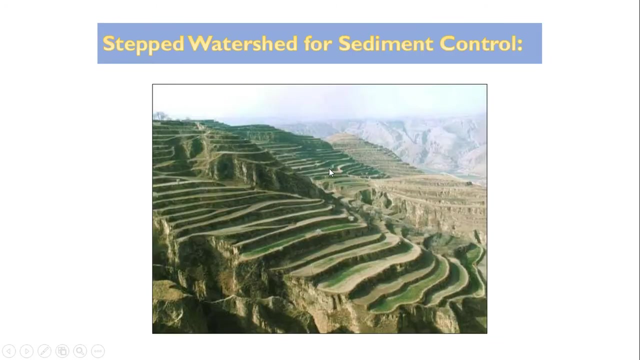 Then this type of nowари can be provided at intermittent level and so that this will obstruct the sediment and there will be sedimentation on this side. so the it is one of the economical way to reduce the sedimentation of the reservoir. sometimes step water step for sediment control is also there. so in case of this type,